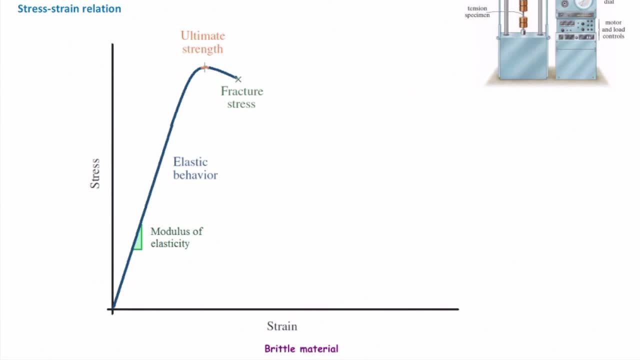 the material. In these materials the fracture happens suddenly after reaching to that maximum load. Let me review this stress-strain curve and see what kind of regions we have in the curve. The very first part of the curve is the elastic region or the linear region In that part. 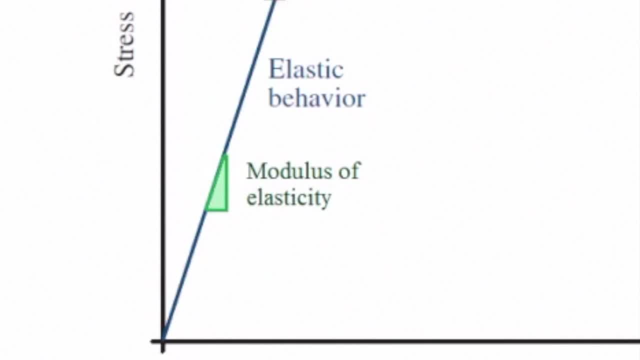 we have two main properties. First, the stress-strain curve is the region where the stress-strain relation is linear. It means that stress and strain are proportional together. So say, if we increase the stress value two times, the deformation of strain increases two times as well. 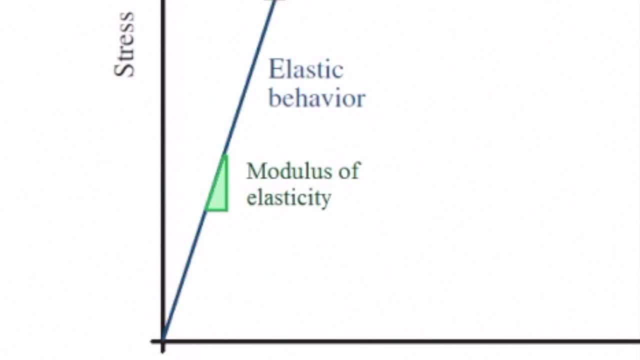 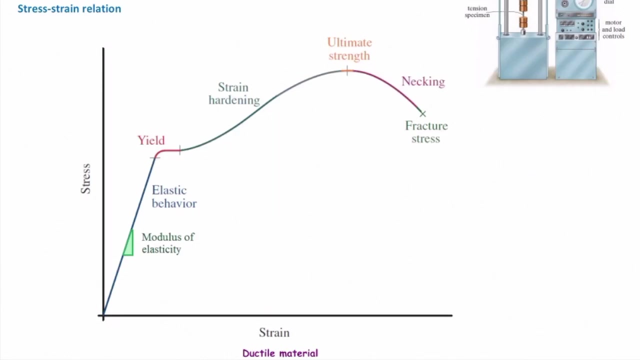 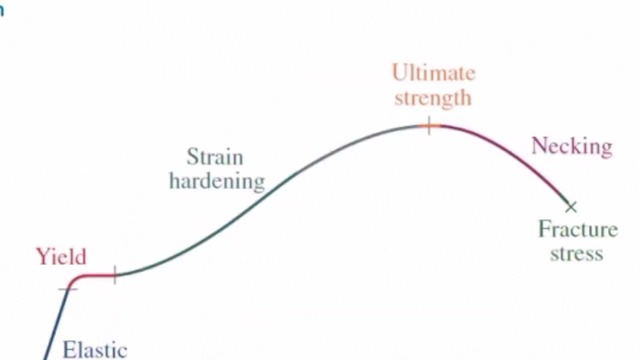 The second important property of this region is if we unload the materials in that region, it goes back to the original point, So there is not any residual strain in the materials. There is a certain point, which we call it yield point. After that, if you unload the material, it doesn't get back to the zero After that yield point. 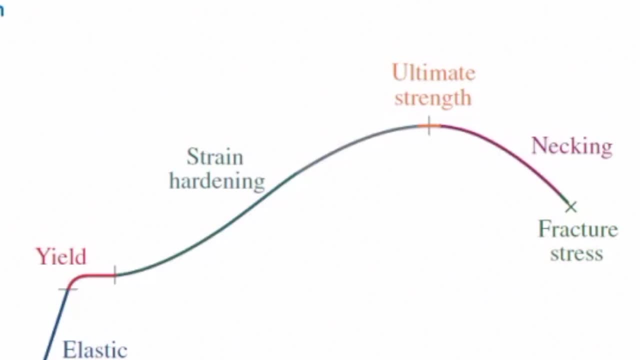 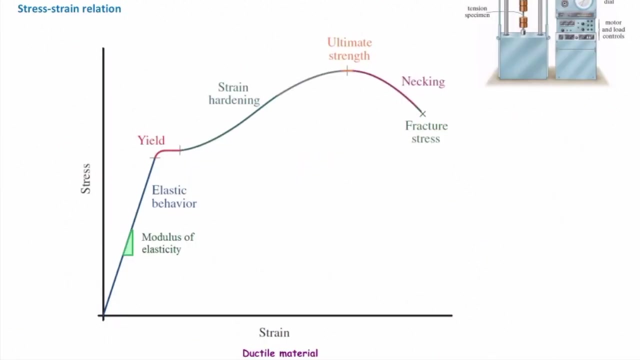 there is usually a flat part And after that there is a hardening part. So strength increases again until reaching to a point, to a maximum point, which is the ultimate strength of the material, And after that we see the failure. This is a typical stress-strain curve for ductile material. 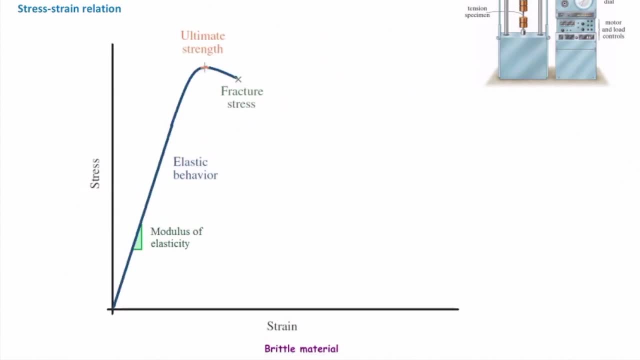 As we discussed, this is a typical curve for brittle material. In this brittle material, we will see again a linear part which has these two main properties: linearity, which means stress and strain are proportional together, and elasticity, which means that if I unload, it goes back to the region. 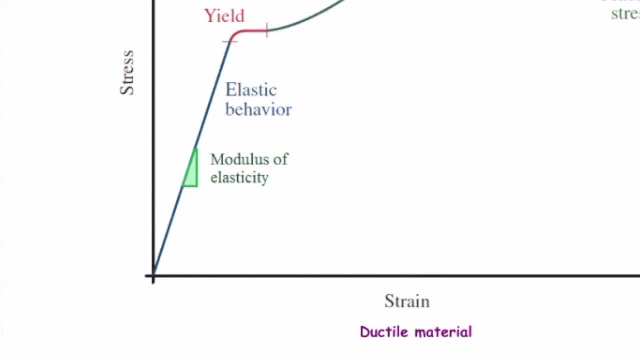 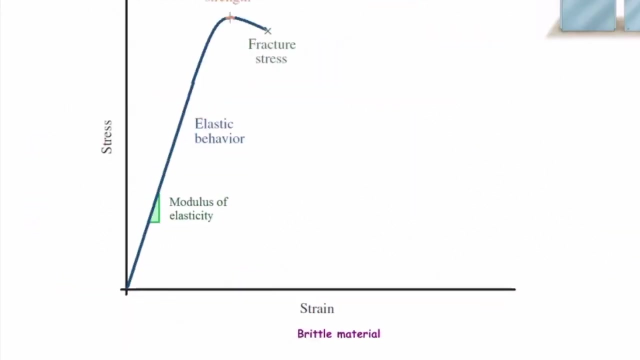 In the mechanics of materials, we just focus on the very first portion of stress-strain curve and we just see this part of the stress-strain curve. In this region we can establish a relation between stress and strain. This is done by introducing a parameter. 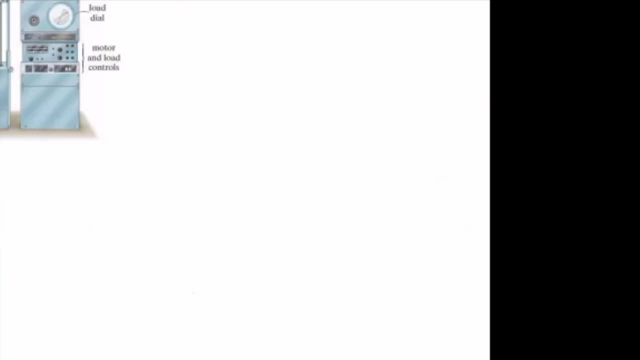 that we call it modulus of elasticity. So what is modulus of elasticity? If we look at the linear part, the linear portion of stress-strain curve, we know that the slope of that line is constant And the slope of that line actually shows a relation between stress increment and strain increment. 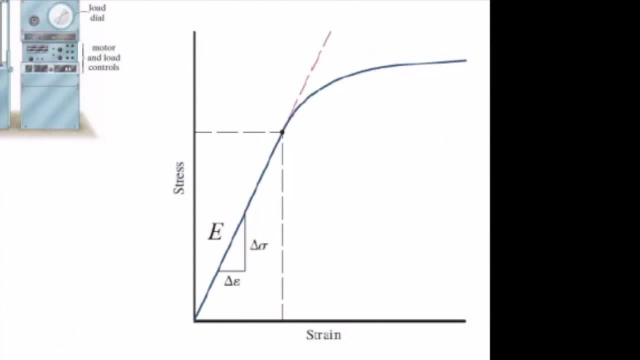 So we will use modulus of elasticity for the decisive stretch of the desenvolvable material onto the structure of blood Hm. So here we can define that slope as the modulus of elasticity of that material. The modulus of elasticity depends on the material we are working on. 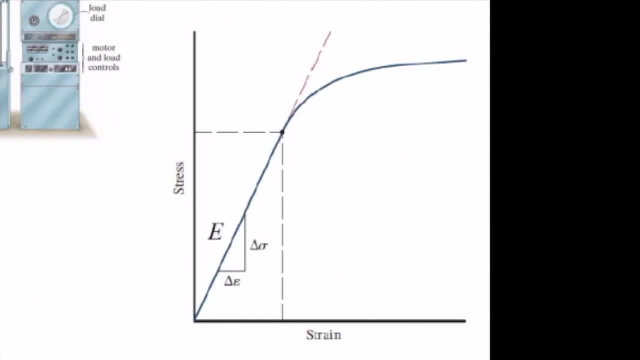 We can determine the modulus of elasticity either in tension or compression tests. For some materials, like metal materials, it is better to do the test in tension. For some other materials, like concrete, it is much easier to do that in compression. Generally, materials have the same modulus of elasticity as description and stress. So all these things are important. units for resonance, 아무뿝م. but we have also seen the세대 파 설. Нет 물건, MAS SEE데, Non audi merci. 응용を 받아 놓은 검사, 모든 wesare는, 모두 정에게 JPN 강력 sharpening'. 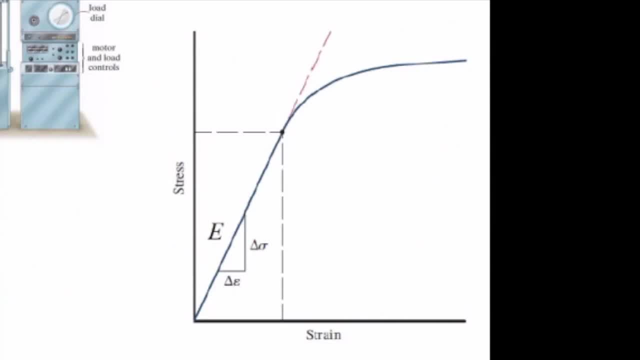 elasticity in tension and compression. There might have different yield points, They might have different strength, but they generally have the same slope either in tension and in the compression. Similar to that, we can define another property which is modular rigidity. 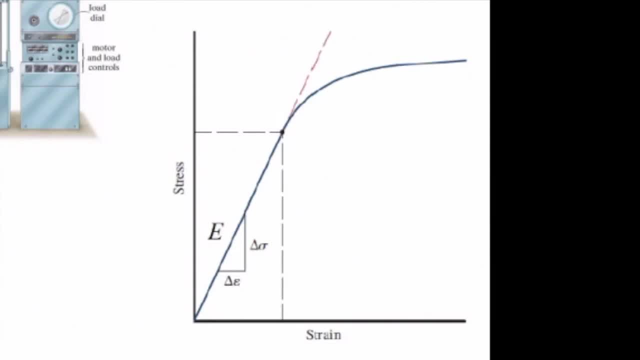 Remember, in definition of modular elasticity we use tension or compression test. What kind of stress is induced in that test? It's a normal stress. That modular elasticity relates normal stress to normal strain. Similar to that, we can define another property which we call it modular. 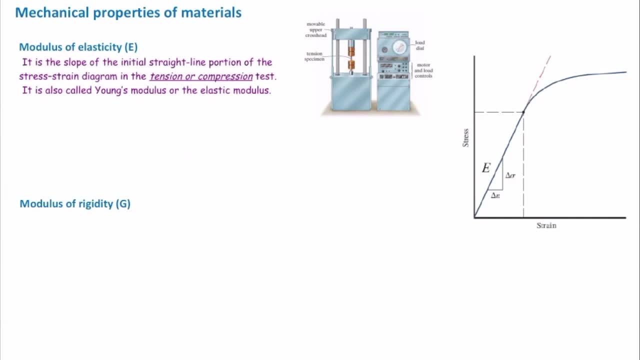 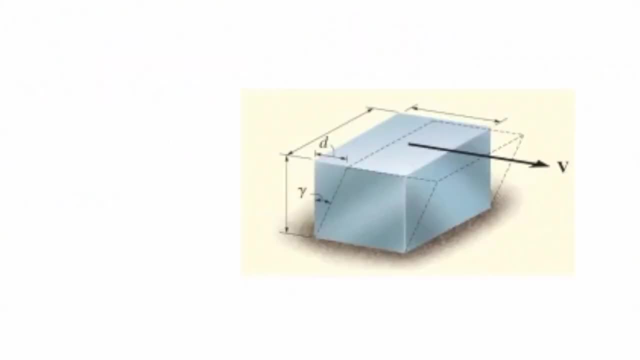 rigidity, which relates shear strain to shear stress. To do that, one way to measure is apply force on the top surface and measure the shear stress caused by that force And at the same time measure the induced shear strain and then try to find a relation between the shear strain and 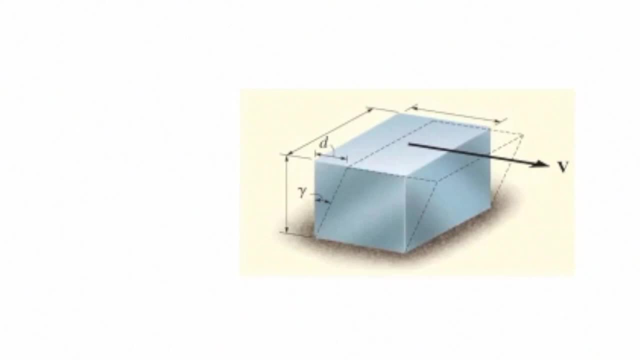 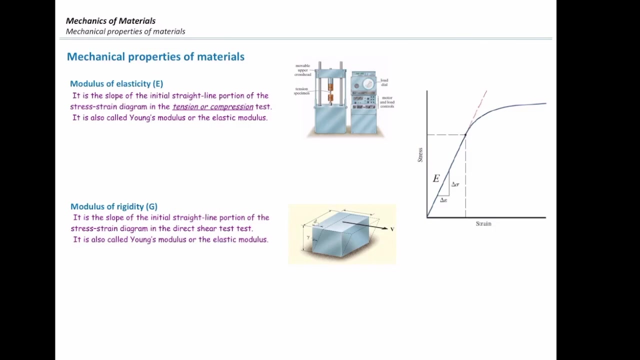 shear stress and determine modular rigidity. This is not a typical test. We usually don't do this test in this way, but we can define modular rigidity in this way. There is another way for indirectly measuring the modular rigidity. So modular rigidity relates shear strain to shear. 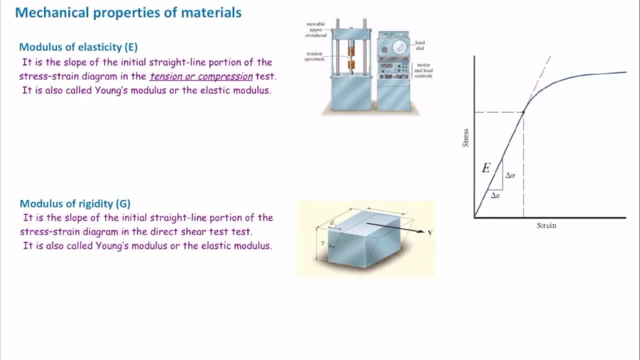 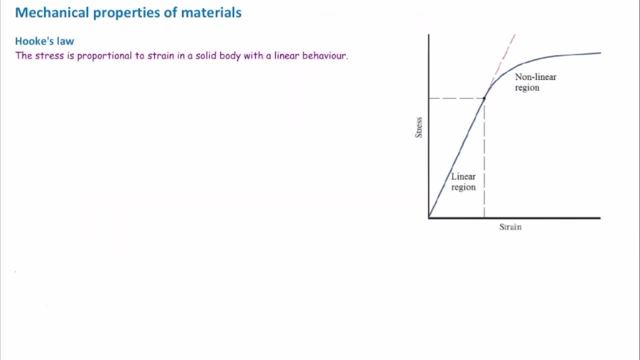 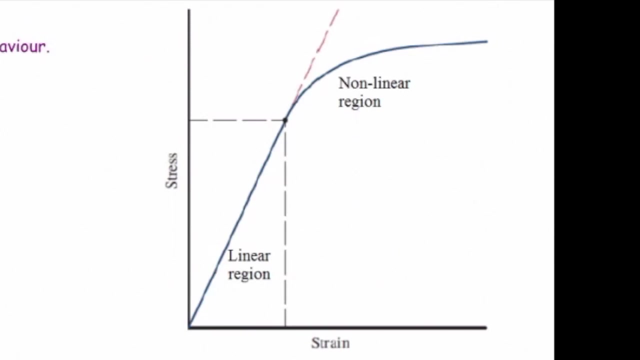 stress in the same way. Let me introduce the equation For relating shear stress and shear strain and normal stress and normal strain. For normal strain and normal stress, we use this equation: Sigma is E, epsilon. If you look at this, E is slope of this line, Epsilon is the horizontal axis And sigma, which is normal stress, is the. 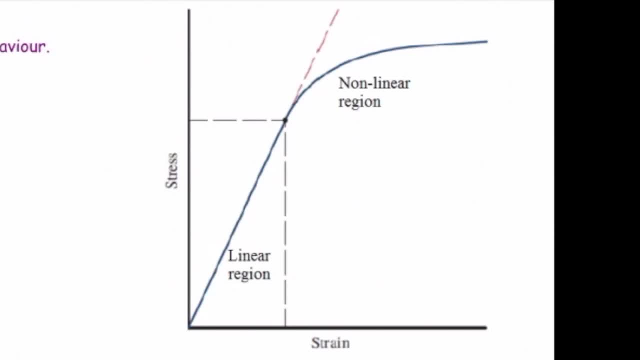 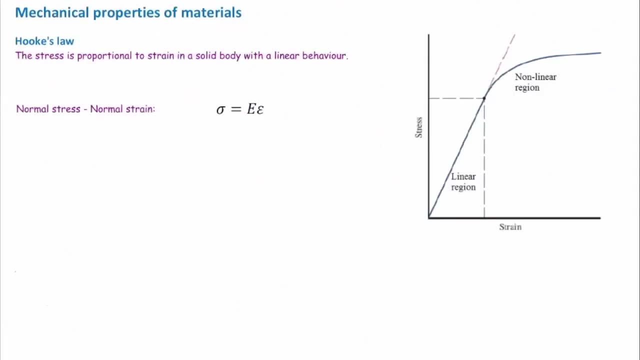 vertical axis. So that is actually equation of a line that passes through the origin. This is what we call it, the Hooke's law. Some of you have done this test for spring in the lab. That is the same equation, so we can define it. the Hooke's constant, which is similar to the modular. 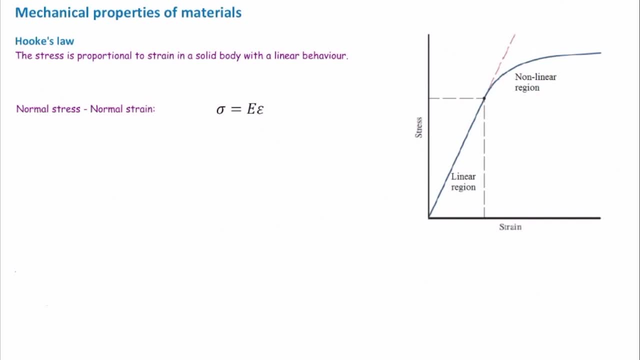 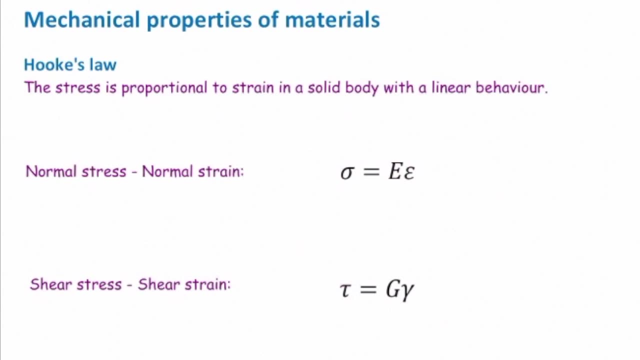 elasticity for spring. Similar to this equation. we can establish a relation between shear stress and shear strain, and that is: tau is equal to G, Gamma G is modular rigidity, tau is shear stress and gamma is shear strain. Ehaba Wafaa Kooz. 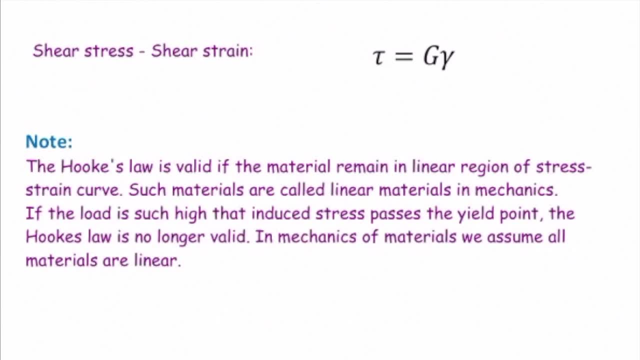 these two equations are valid if we remain in the linear region, which is the case in mechanics of materials. If the stress is high that causes passing through the yield point, we can't use these two equations anymore. But in the mechanics of materials we assume that all stress levels are below the yield. 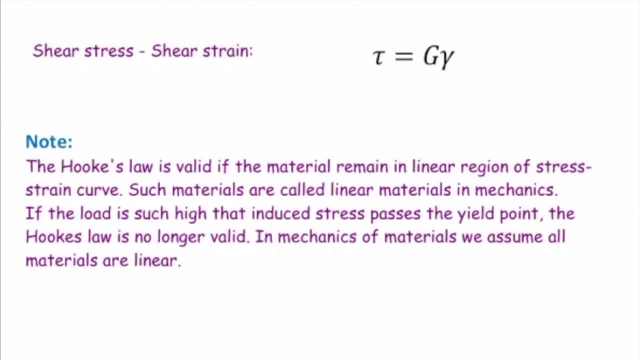 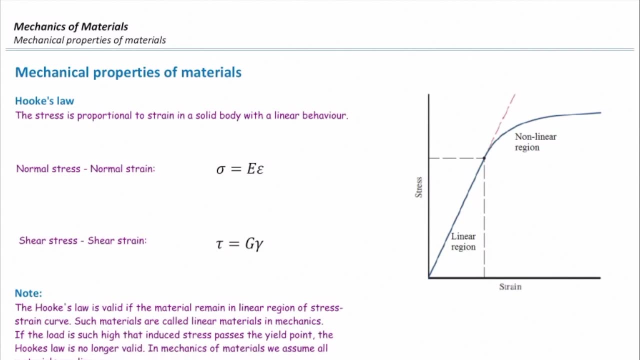 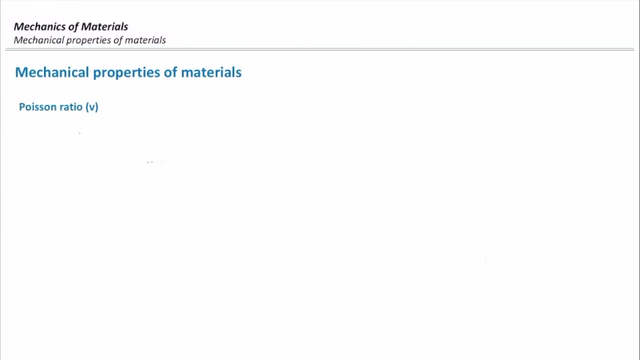 point, so we can use the Hooke's law for relating stress and strain together. The last parameter, the last mechanical properties parameter that I want to talk about before solving a problem, is the Poisson ratio. What is the Poisson ratio? Let me explain it in this way: Consider that you have a piece of sponge. What? 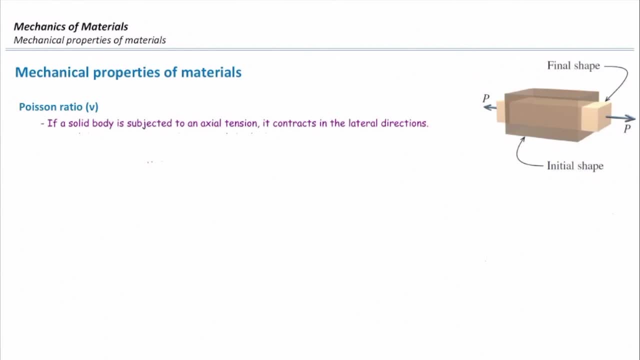 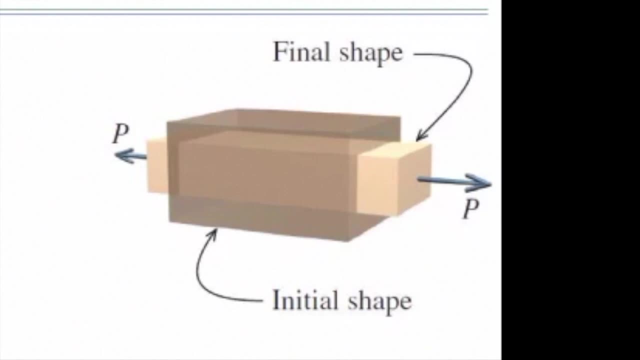 happens if we put tension on that piece of sponge that stretches, So we see increment in the length. Is there any change in the length of that sponge perpendicular to the longitudinal direction on the sides? What happens? What happens in that case? It shrinks. Okay, Similar to what? 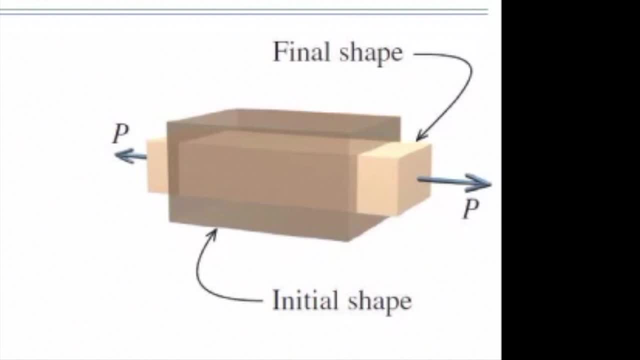 we see here. so if I apply load in that piece, this is the initial shape and this is the final shape after providing the load That stretches in the longitudinal direction and that shrinks on the sides. This is what we call it Poisson effect. 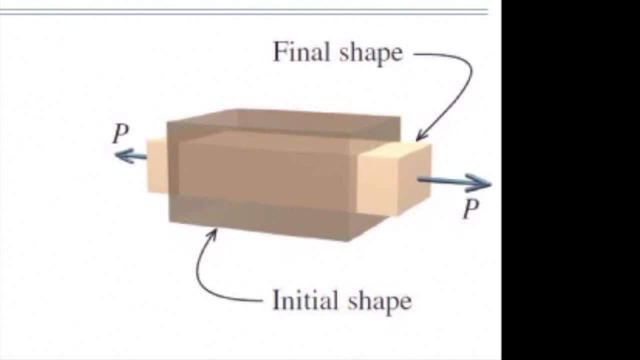 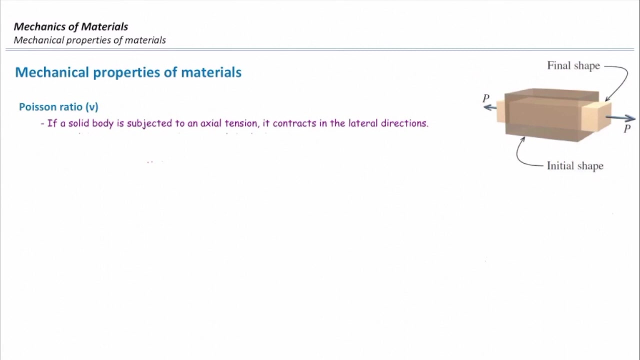 So by applying the force in one direction, we don't see strain in that direction only, but we also see a strain on the perpendicular direction, only in the lateral directions. This property was first noticed by a French mathematician whose name was Poisson, and this parameter is named after him as the Poisson ratio. Similar to that, we can do the 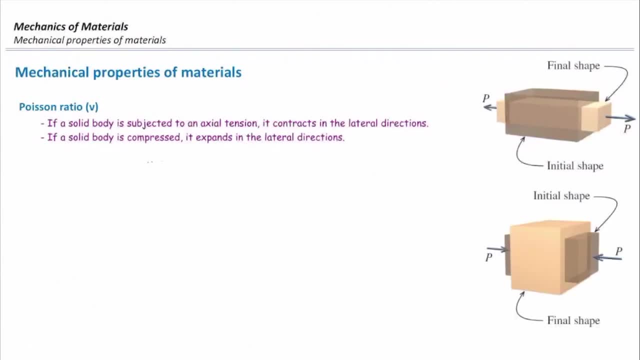 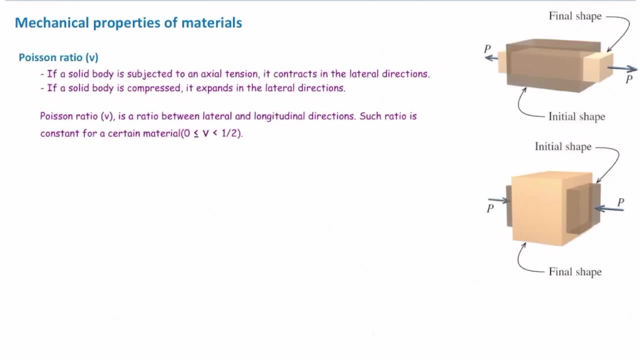 test in the compression. So if you compress one material that expands on the sides, on the lateral directions, The Poisson ratio is typically 0.2, 0.3 or something like that. in the different materials The minimum possible value is zero, It can't be negative and it can't be higher than 0.5. 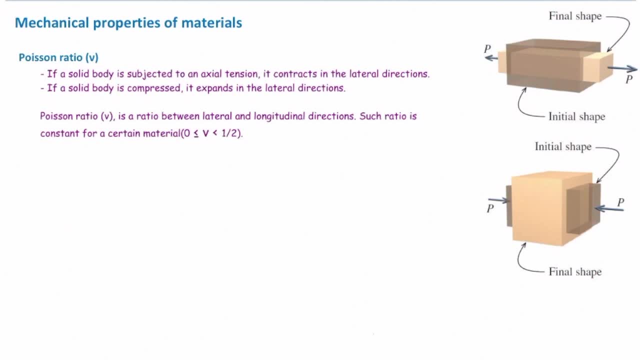 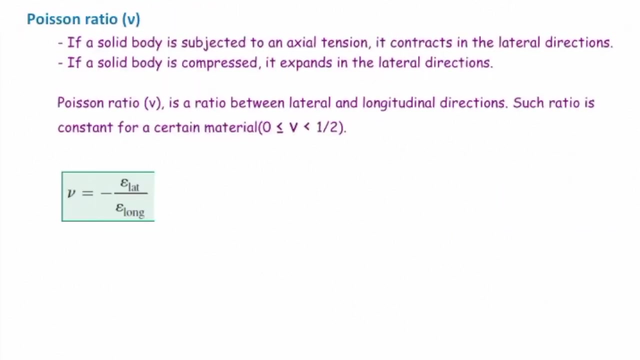 It is impossible to have a Poisson ratio higher than 5. and negative is impossible because when you put tension on the element, it is not expanding on the side, It is shrinking on the side. so it can't be negative. The equation for the Poisson ratio is this: one Poisson ratio is shown by nu. It's a Greek letter. 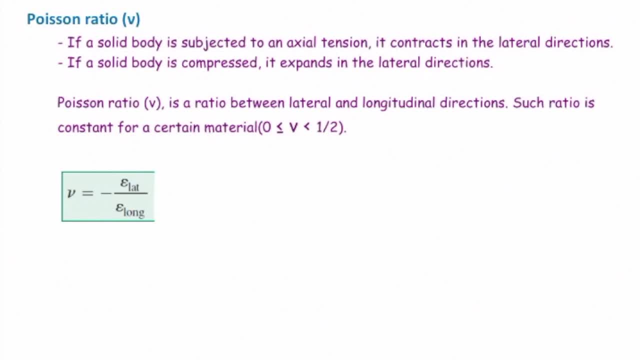 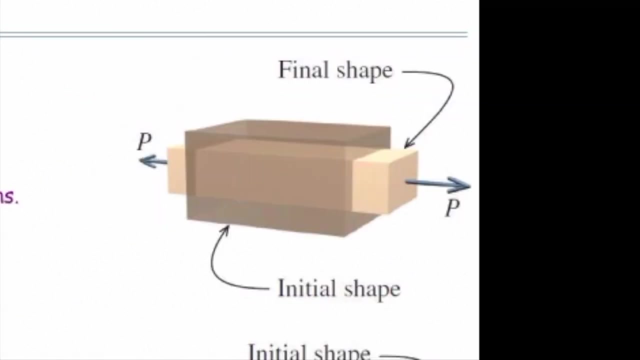 and is obtained from this equation: Strain in the lateral direction divided by strain in the longitudinal direction. Longitudinal direction is the direction of the applied force and the lateral direction is any direction perpendicular. So for this case, the horizontal direction is longitudinal and the vertical and the direction perpendicular. 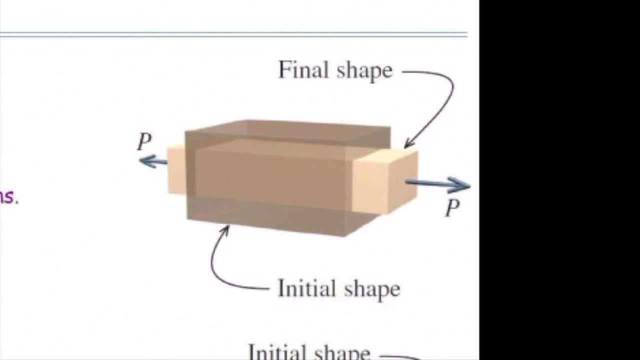 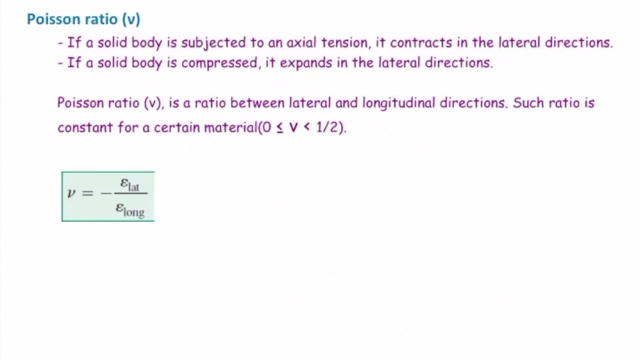 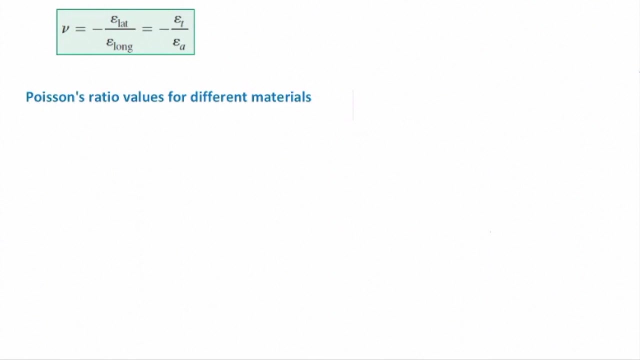 To this plate is lateral direction. Here we used a negative sign. Why? Because if longitudinal strain is positive, the other strain is negative. To have the Poisson ratio positive, we use a negative sign in this equation. The typical values for Poisson ratio are given in this table. 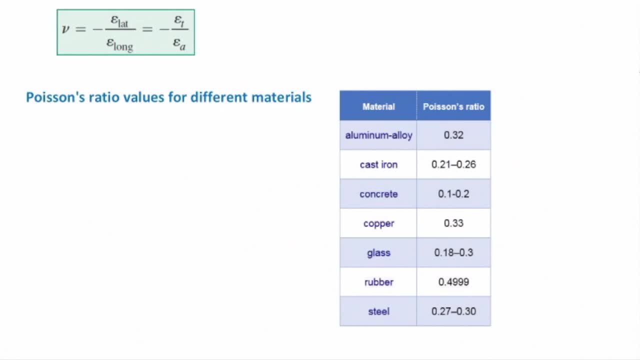 For steel it's typically 0.3, 0.25, 0.25 and 0.0.. 0.25, 0.27, 0.23.. For concrete it's a bit lower. It's 0.1, 0.2.. The highest typical. 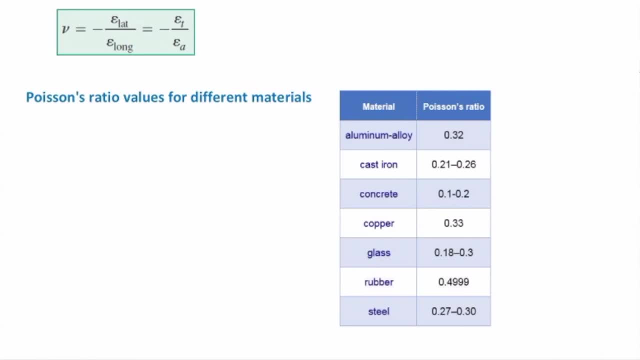 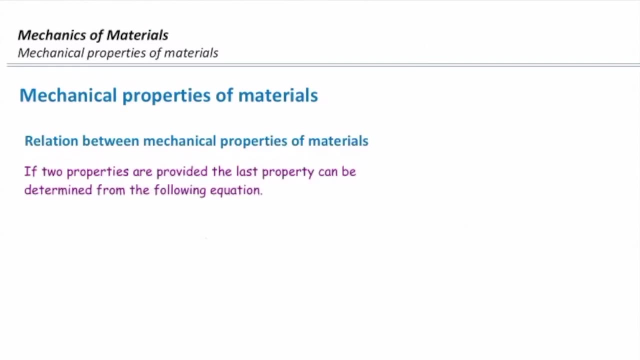 value is for rubber, It's 0.4999.. It's very close to 0.5.. So we have introduced three parameters: module of elasticity, or E, module of rigidity or G, and the Poisson ratio. 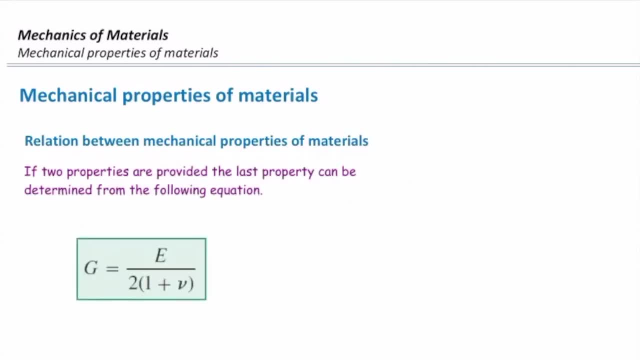 or nu. We can relate these three parameters together using this equation. It means that just two out of these three parameters are independent. In other words, if you determine two of them, you can determine the third one. So the typical way to measure module of rigidity.